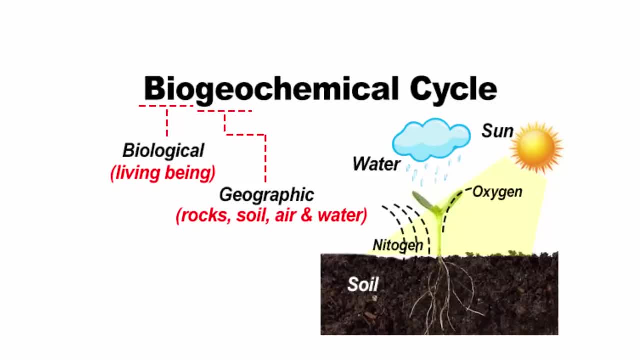 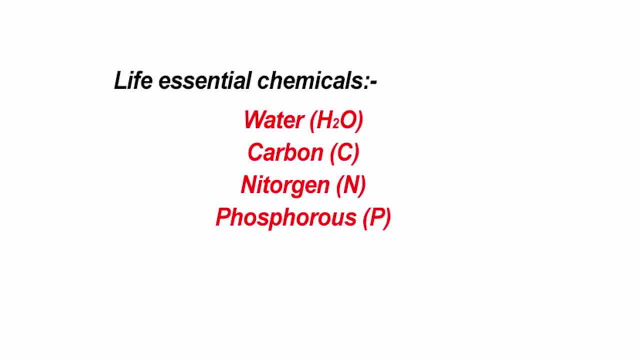 chemicals that are present in the environment that determines life on earth. Can you think of them? Water, H2O- It is important right. Then we have carbon, Then we have nitrogen, Another one is phosphorus. There are many more, but these are some important chemicals. 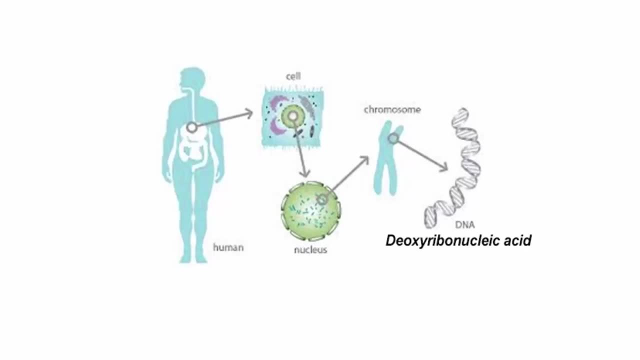 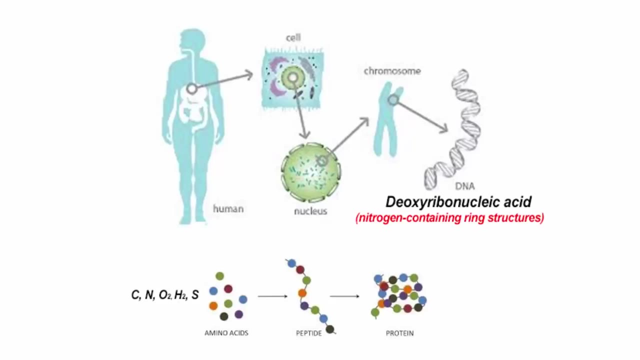 Now look at the following. You have DNA deoxyribonucleic acid. It contains nitrogen molecules. Then your body needs amino acids, which are essential nutrients for the body to function, And amino acids contain carbon, oxygen, hydrogen, nitrogen, sulfur, etc. Your bones contain phosphorus. If you look at carbon, 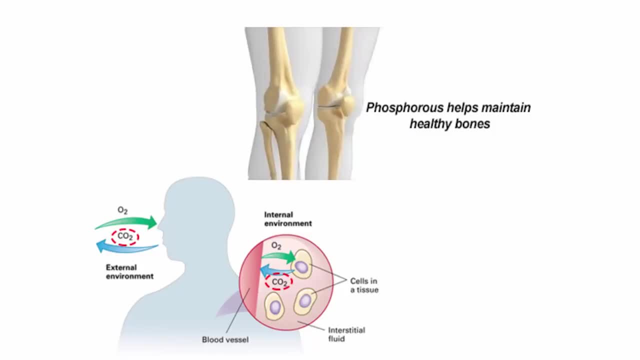 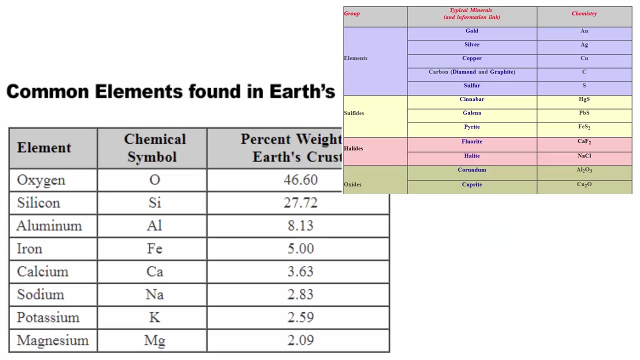 it is the basic building block to most cells in the body. It helps with cellular respiration, by which your body releases energy stored in glucose, and glucose compound is composed of carbon hydrogen and oxygen. You see, these are essential chemicals for life. Now these same chemicals are also found in rocks, soil, air and water. 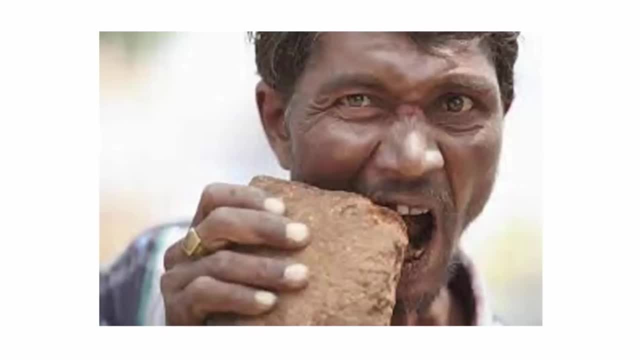 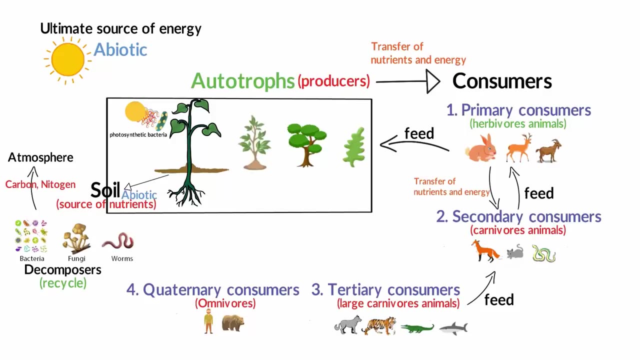 But it doesn't mean that you start eating rocks and soil directly to have these chemicals in your body. Rather, these chemicals from the environment goes through a process and turns into food. We have talked about this when we read about the structure of the ecosystem: how one organism 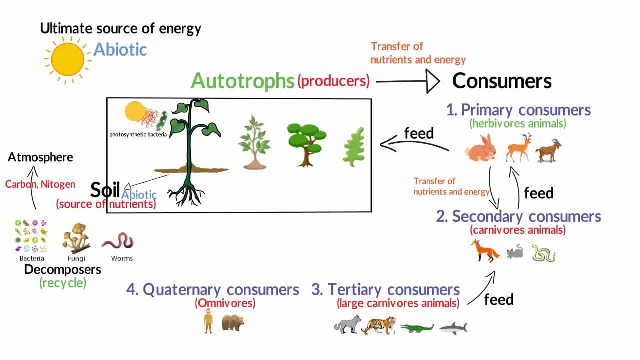 eats, another for food and energy. That's how energy gets transferred from one form to another, While some of the energy gets lost in the process, but essentially, these important chemicals get recycled. And if you see, most of these chemicals were present during the initial time when the earth was. 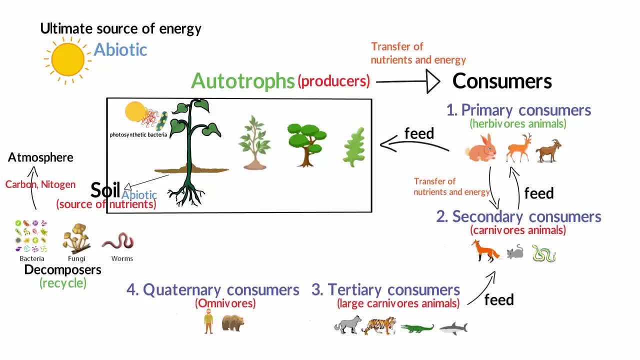 formed. That's why we call them as life essential chemicals. Anyhow, these chemicals go through a process and turn into food which you are able to consume, and that's how your body is able to function and have these chemicals replenished within you. 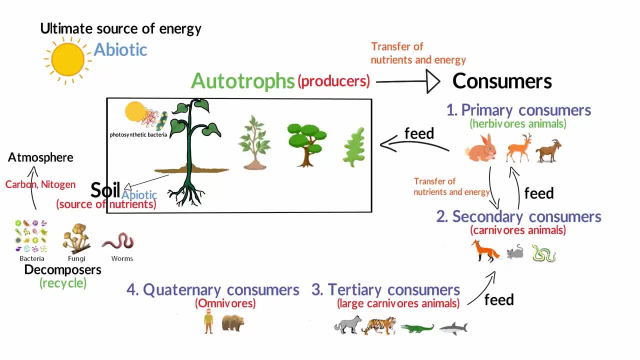 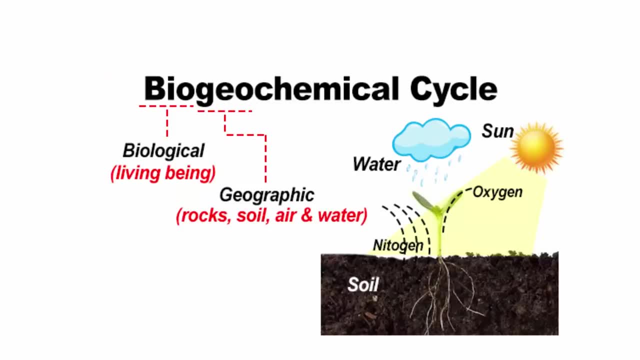 After you die, all these chemicals are returned into the air, water and soil through decomposition. So this entire cyclical movement of chemicals between the abiotic and biotic components of our environment is referred to as Bio geochemical cycle. 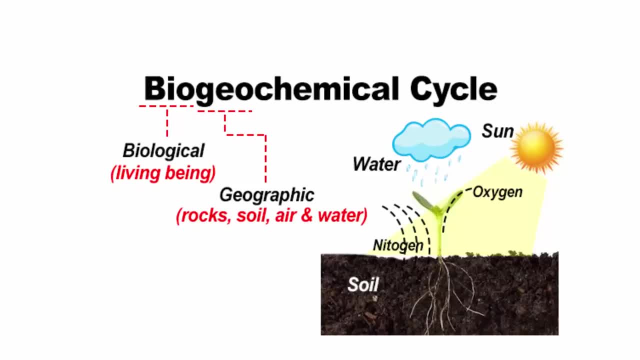 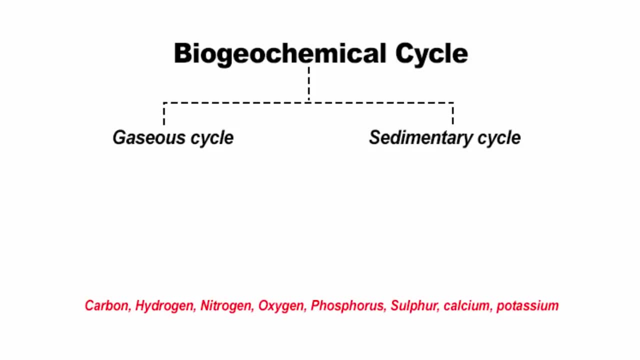 Now that you have understood what a bio geochemical cycle is, you have to understand that it is of 2 types. The reason why I said it's of 2 types is because, if you look at the important life forming Vital Chemical Elements of spartan acid in this cycle is 10.2 milion Milton.